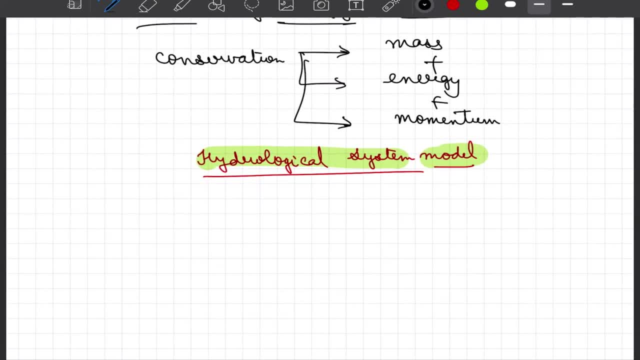 in context of hydrology we define system or a hydrological system as a structure or volume that has some finite boundary, And these boundaries they will take some input in form of water, energy, air, do some manifestation on it, So some water may go. 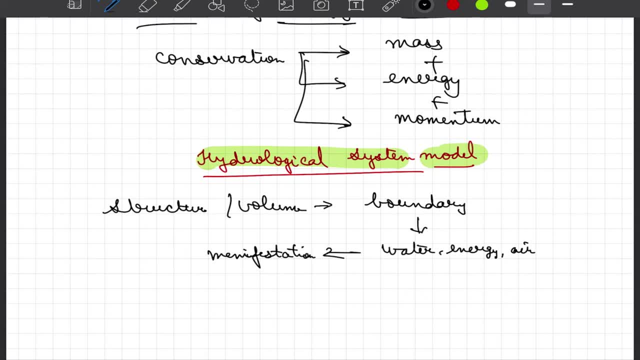 as groundwater. some will stay intercepted, some would be retained by crops and so on, And after this manifestation has happened, we will have some how to define hydrological system. So we will try to understand how to define hydrological output, which would be, let us say, discharge, And this entire assembly of these components. 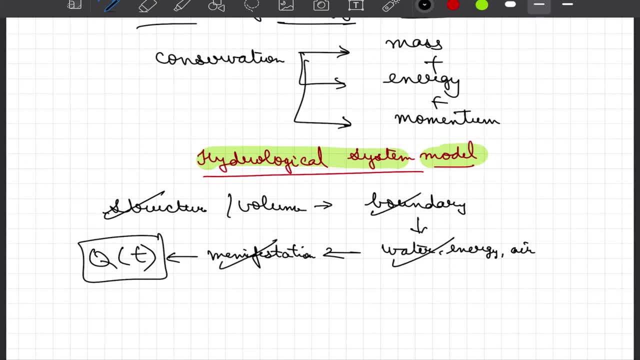 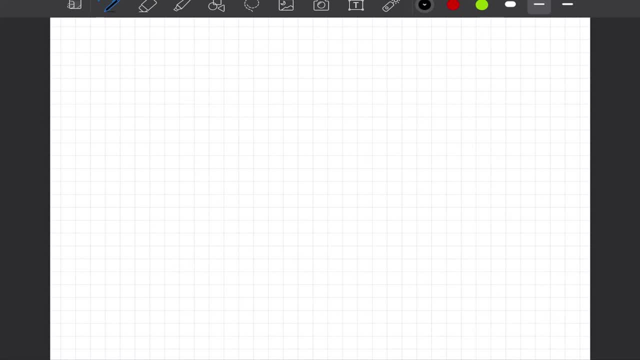 that is, structure, boundary, inflows and manifestation, is called as the water hydrological system. Now let us also. another important term that we will encounter frequently is the watershed. So to understand watershed, let us try to see that with help of an example. 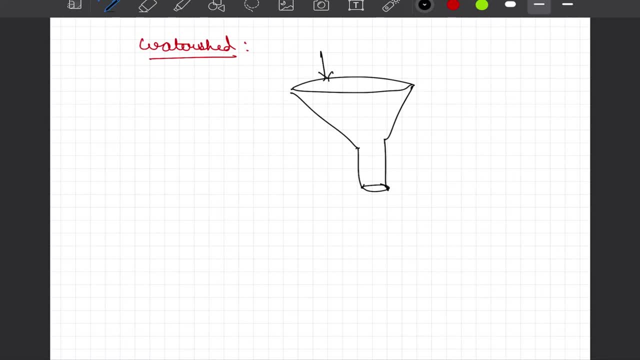 Let us consider a funnel and this funnel will take some inputs as I- t and there would be some outputs as Q- t. In a real world, watersheds are similar structure. that means that whatever is falling in or falling onto this area, that will stay within this particular funnel and everything. 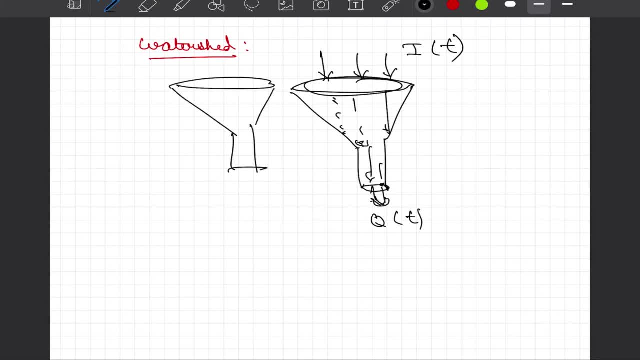 else would go to the second funnel. So there these watersheds are going to have the watershed lines which we call as watershed divides. That means everything falling within that divide belongs to that watershed and everything falling outside that divide belongs to another watershed. Now, if you have to put a boundary, we should put a boundary in a way that 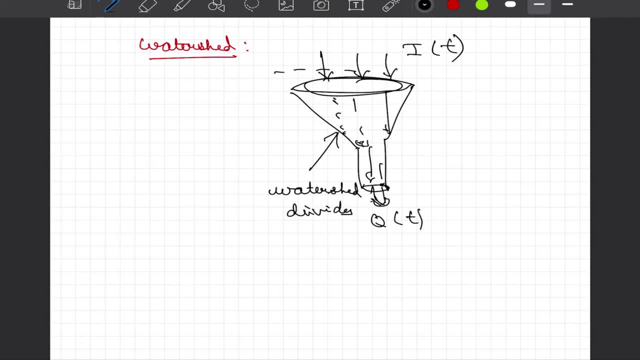 all the influxes and outfluxes are accounted for. So we will choose boundary strictly, in a way that we are not missing any path line from where we are going to have the watershed lines. So let us consider a funnel, and this funnel will take some inputs, as I t, and there would be some outputs. 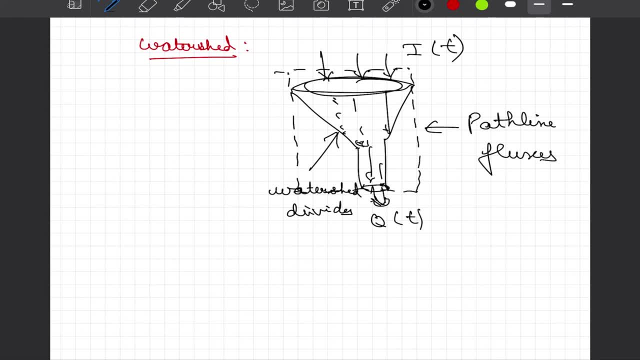 as I t, and there we could have some possible fluxes of water, air and energy that we just mentioned. So now we clearly see that and since this funnel would be a three-dimensional object, this shape that is enclosing it, it has to be a three-dimensional cylinder. and when we are dealing 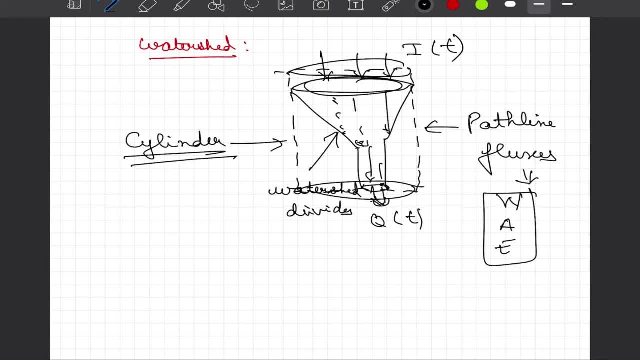 with cylinder, we are dealing with a specific shape which has a boundary, and there would be certain manifestation occurring here. And in case of a simple funnel, this manifestation would be: whatever is coming in, that is going out Now. but now you get little bit more adventurous and say that I will plant some small plants. 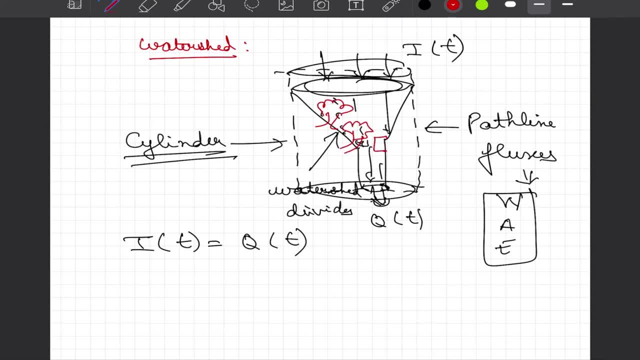 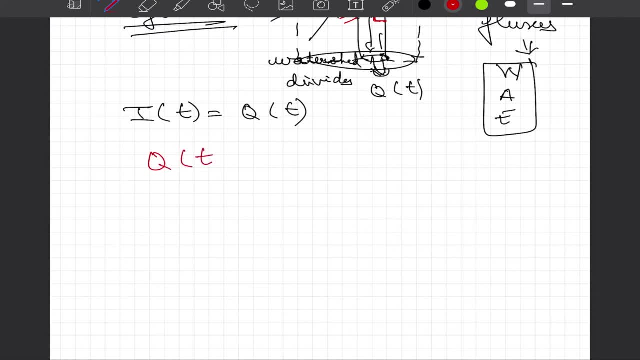 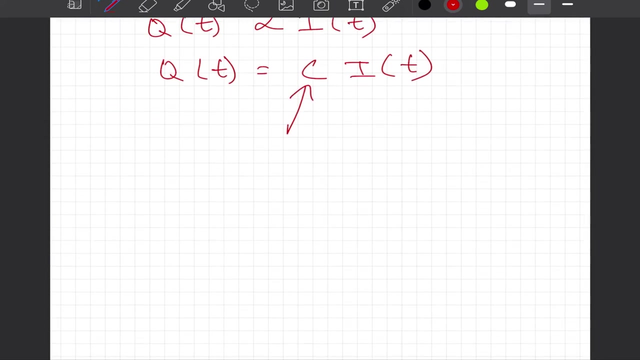 or I will design some retaining structure in this particular funnel where I should be able to store the water. That would mean that now your Q t would be proportional to I t, and this would be related by some constant C. So what we are going to do is we are going to take this Q t and I t, and one of the purpose of 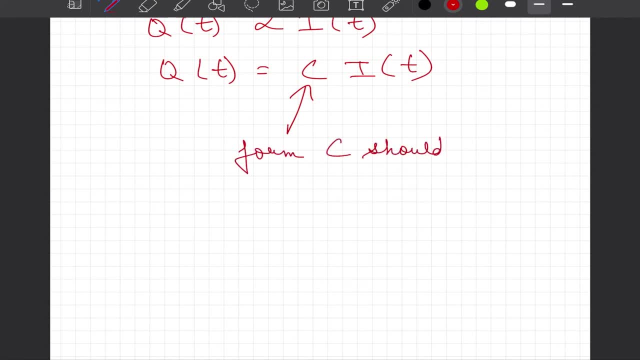 hydrological model is to determine what form this C should take, so that we are able to tell how our output is going to look like. So essentially, it becomes a predictive model. if we are talking about a stochastic setting, where idea is, given certain sets of inputs, what is going to be an output? 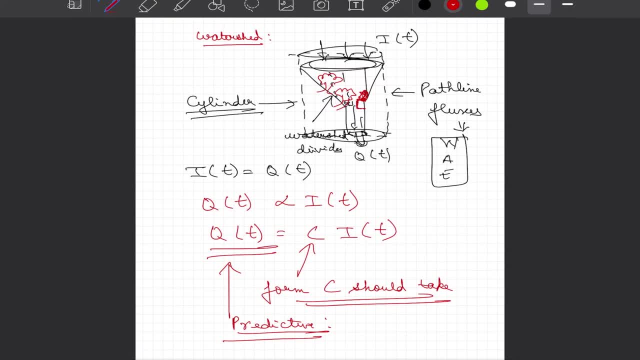 And we are going to study this output in a very specific way, And we are going to study this output in a very specific way. However, we are going to study this output in a very specific way, So in a real hydrology. our examples are not going to be as simple as this funnel, But whenever the 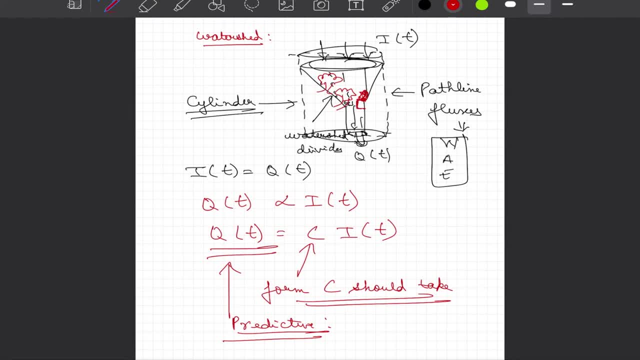 concept of watershed comes. always remember that within a funnel we will have a certain structure through which water will flow, certain manifestations will occur And at the end we are interested to tell what is going to be the output. And we will study this output dedicatedly in the 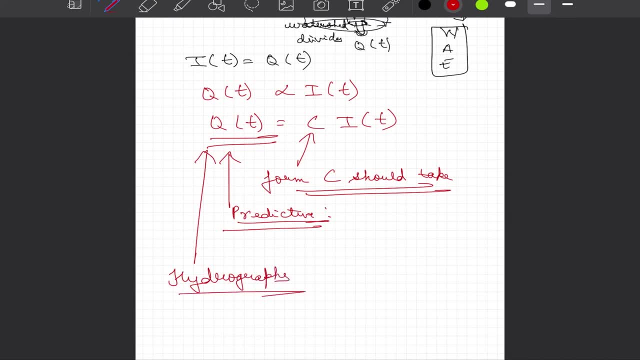 form of hydrographs. There would be a dedicated units to study that, how this inputs manifest and how basin or watershed corrects it, And we are going to study this output dedicatedly in the form characteristics control these hydrographs, which in turn would determine how much flooding we are. 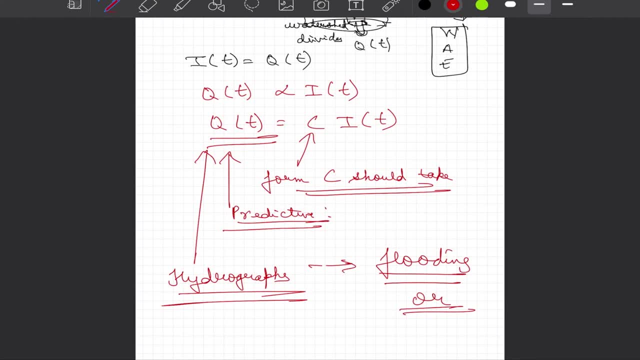 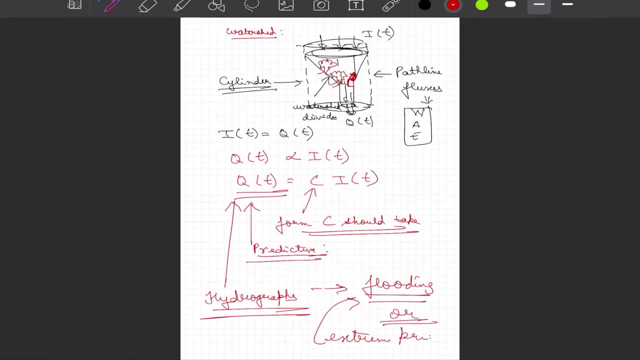 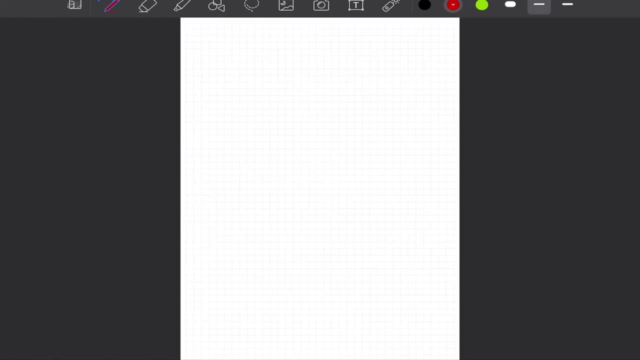 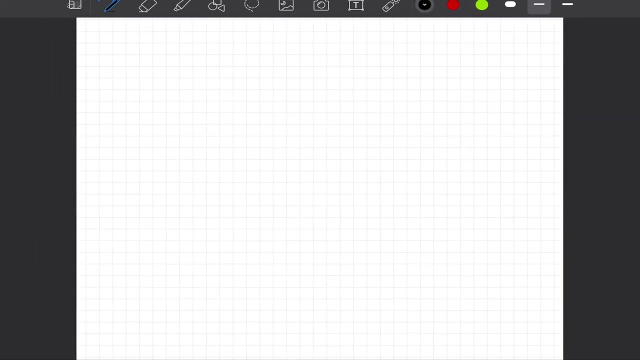 going to receive and how much of the extreme precipitation will manifest into flood levels once we determine these hydrographs. Now one thing is clear: that we are going to abstract a very complex system into some simpler representations and we call this entire construct of simplification of a complex real world system into simple representations as hydrological modeling. 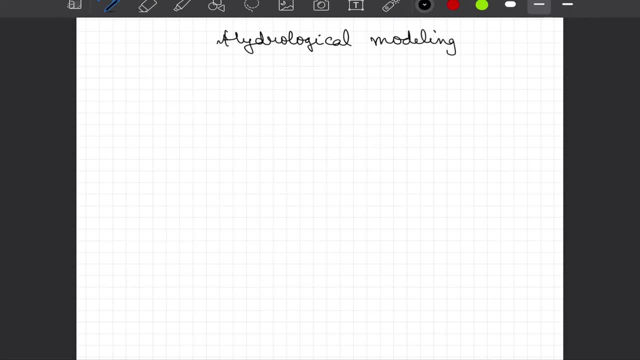 So now let us look into the aspects of hydrological modeling. So hydrological modeling would essentially deal with determining what is the relation between input and output, and we can have two kinds of hydrological models. As models try to simulate the reality, we can have some physical models, small scale, hydrological. 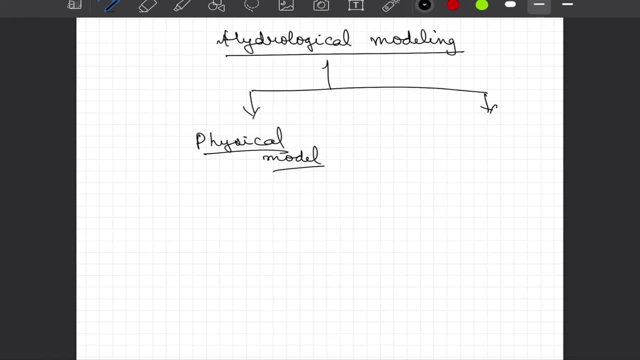 model. So the model that you have in IIT Gandhinagar hydraulics lab, it's a physical model which represents a small watershed on which we simulate an artificial rain and the discharge happens, and these are the experiments that you will do in your laboratories. Similarly, we can have the abstract: 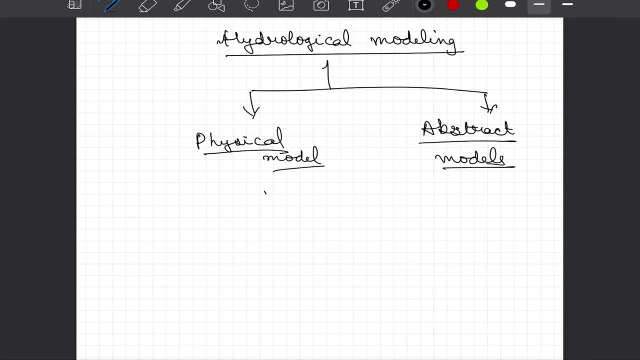 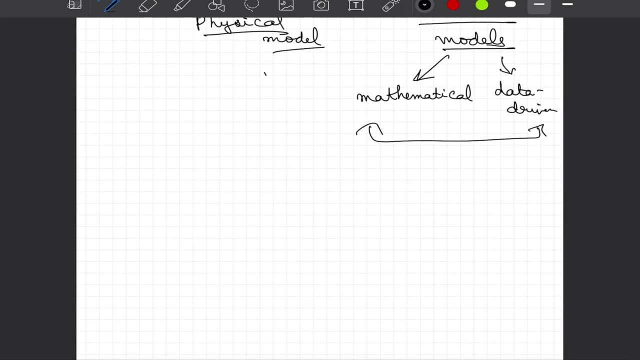 mathematical models that are based either on certain mathematical principles, such as conservation of energy, conservation of mass, conservation of momentum, or they are purely data driven, And we will be primarily dealing with the abstract models in the context of discussions that we are going to have given. 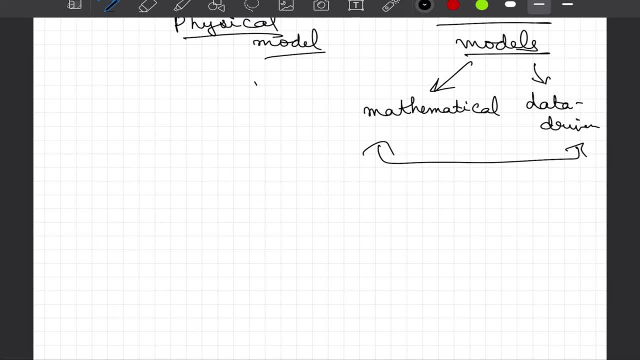 there are certain benefits because they are scalable. they are easy to comprehend and solve, using pen and paper as well, as you can model a small watershed of few square kilometers As well as large Amazonia river basin, which is in few hundred thousand km. Now, we can also have a different level of complexity associated with these models. 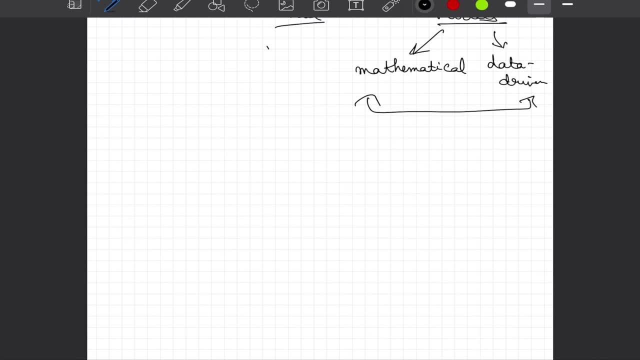 For example, again consider IIT Gandhinagar as our area of study. You can say that within IIT Gandhinagar we would have precipitation of different intensities happening in different parts. for example, if we have student hostels here are academic block here. 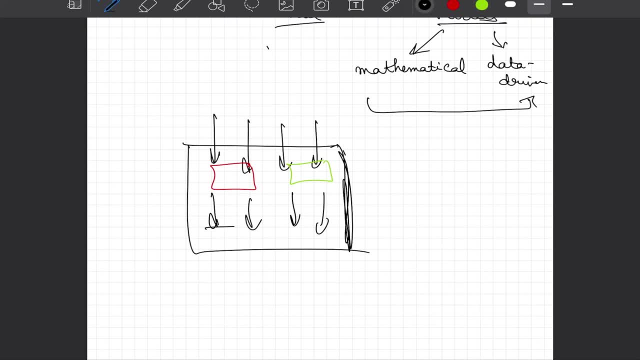 or primitive bibelte del��면 building, see IIT Как defeat, as you can see our faculty housing here. there is high likelihood that these three areas may receive at same time different intensities of precipitation, So I1t, I2t and It3, such that 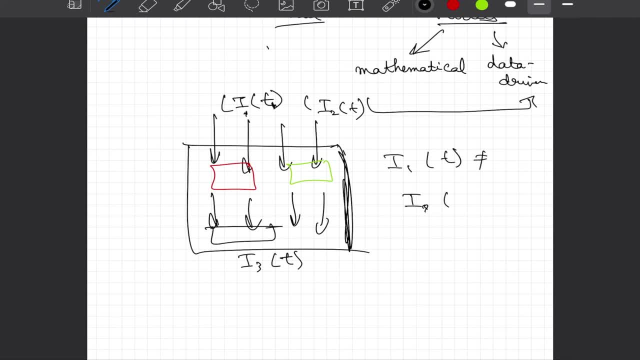 the intensities of precipitation are not equal in many cases, But you do not want to model these system as at much finer resolution, But you do not want to model this system at such granularity. So you would say that I want to lump this entire campus and we will use an 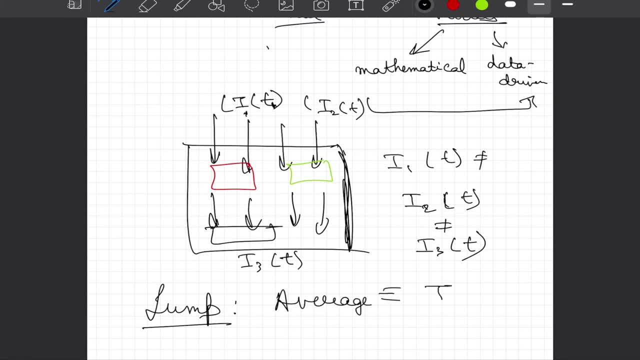 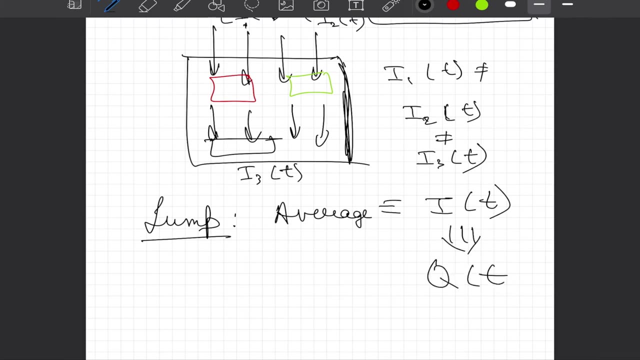 average precipitation And this average precipitation is represented by, let us say, It3. That is, the average amount of precipitation that has taken place over IIT Gandhinagar campus is represented by It3.. Also, you are interested to look into how much discharge would come out. 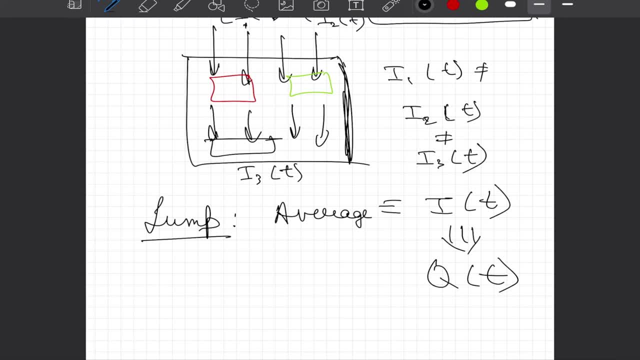 of the IIT Gandhinagar. If we consider this, IIT Gandhinagar is a funnel, in a way that everything will go out to one specific point and you are interested to model this Qt. Now, what you would need here is that you are averaging Qt, you are averaging I, and you would say that I will represent. 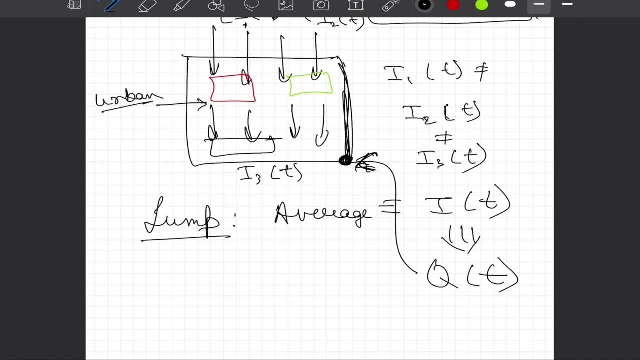 this IIT Gandhinagar as an urban form. That means there is a lot of concrete and I have calculated that, on an average, 70 percent of rainfall will run as runoff. So what you have done, you have lumped all the physical properties of such a big area into one representative number and you say: 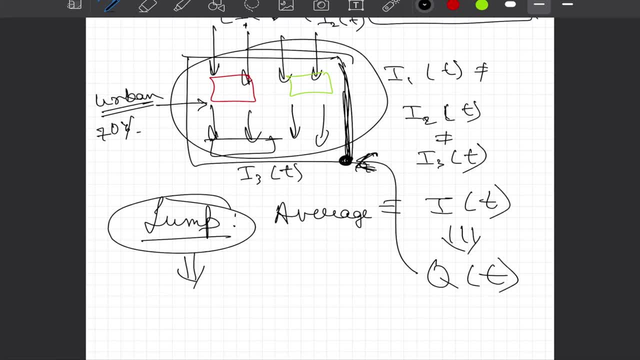 I will apply the conservation of mass momentum, energy and so on to estimate this relationship between Qt and IIT. So you are basically looking at the lumped model- These are called as lumped hydrological model- where you represent an area of non-zero magnitude as a dot or as a point, and 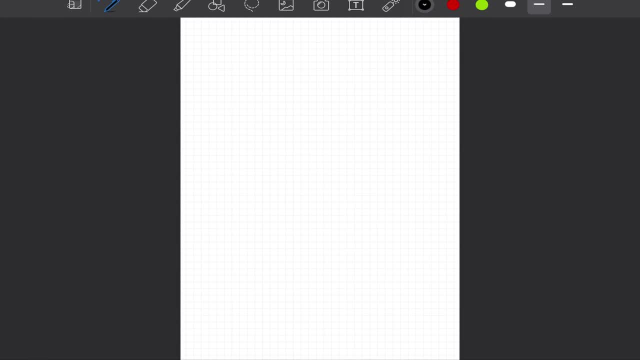 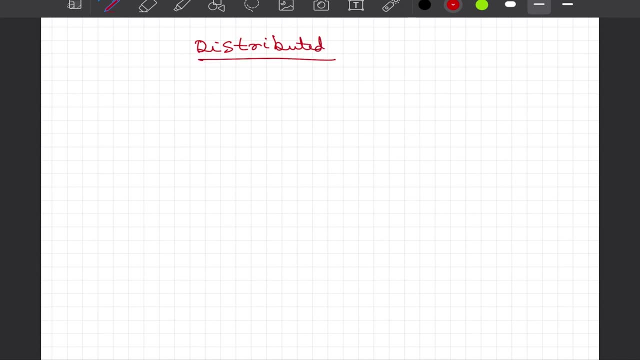 concentrate all the properties there. Similarly, you can define a distributed model. You would say that now, instead of modeling IIT Gandhinagar as one single dot or one single unit, let me divide IIT-GN campus into large number of small grids, and these grids, basically, would: 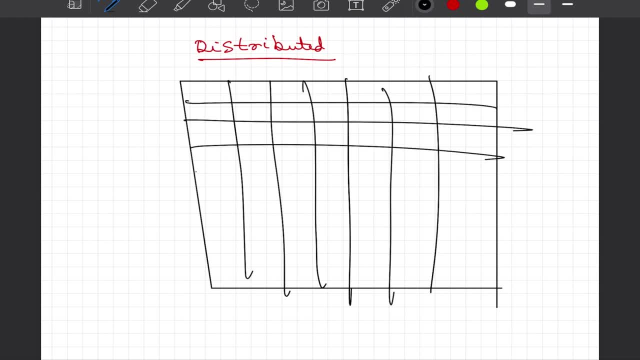 all of these grids have different properties. that would mean that if there is a green patch here where students play foosball or or any other game, that would have a green patch. on the other hand, our hostels- they would be primarily concrete and hence would be represented as black. 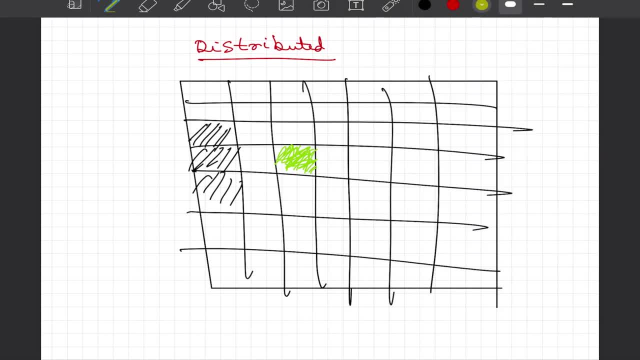 patch. on the other hand, if you talk about the faculty housing area, that would be mix of both green patch as well as concrete patches, and so is the case with our academic block. now you have basically decentralized the properties and you will say that for concrete and I will use a different coefficient, and we will talk about these parameters later on.